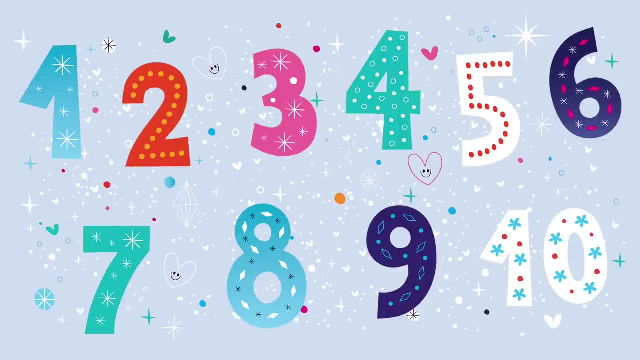 Listen to your breathing. Can you hear it coming in and going out? See if you can slow it down, making it come in through your nose and out through your mouth. That's it, Gently: in through your nose and out through your mouth. 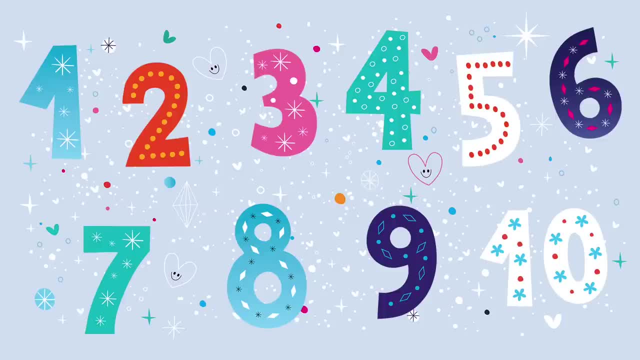 And this next time, as you breathe out, gently close your eyes. Lovely, Now let's try something with our breathing. A game, I wonder if you can count your breaths. Let's try: As you breathe in, you count one. 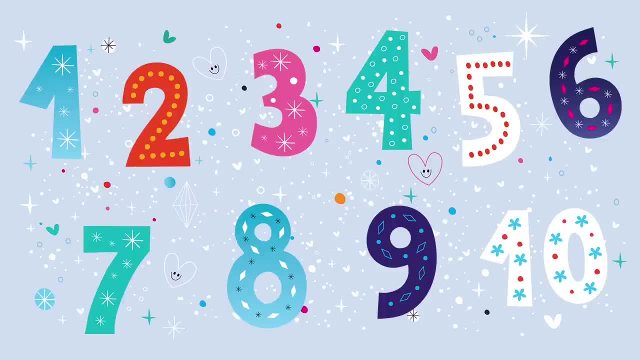 As you breathe out, count two. As you breathe in again, count three. And as you breathe out, again, count four. Can you keep counting the in and out breaths all the way up to ten? Maybe this seems too easy. It will be if you breathe fast. 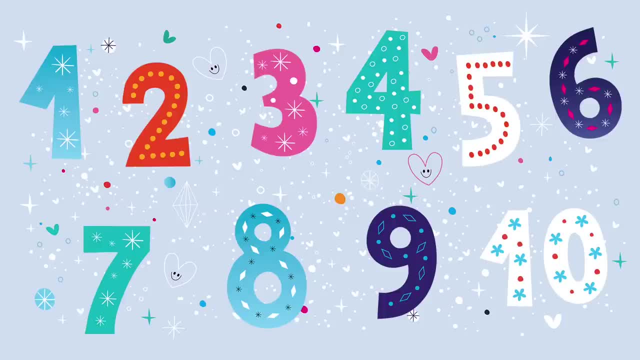 So can you try and breathe slowly and do it? The slow way is the more advanced, harder level, But I reckon you'll be able to do it. When you've counted up to ten, make your next breath one again. The challenge is to see how many sets of ten you can count. 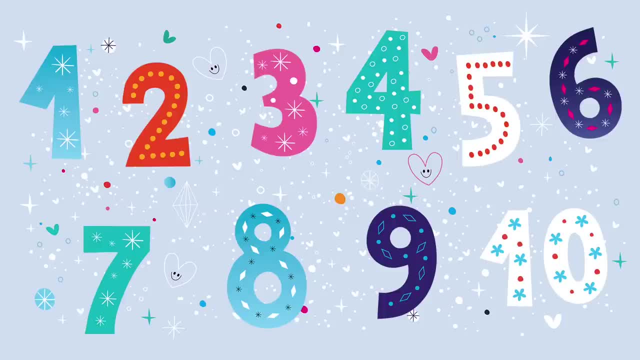 Each breath in And each breath out is a count. If your mind wanders off and you've found you're thinking of something else, don't worry. That's great because you've spotted it. If you do spot it, see if you can just bring your mind back to your breath, starting at one again. 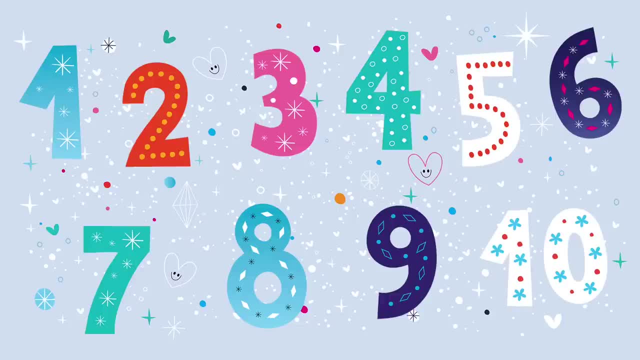 I'll give you some space now to breathe and count, Count. I haven't gone anywhere, I'm still listening to you. You're doing really well. Just so. you know, grown-ups find this really hard, So if you're doing it, then you're doing an amazing job. 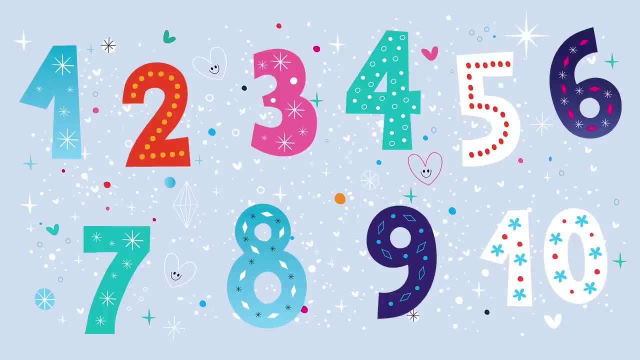 Thank you. Now, wherever you are in your counting, just let go of it and let your mind wander off wherever it wants to go. You can think of anything you like, just let the thoughts come back in. Well done you. that was really good. 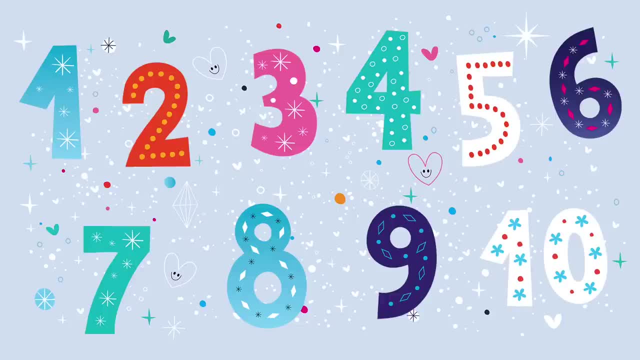 It's time to start bringing yourself back to the space you are in, Feel your body where it meets the floor or chair underneath you, Hear the sounds around you, those close by and others far away. Take a big, deep breath in and sigh out of your mouth. 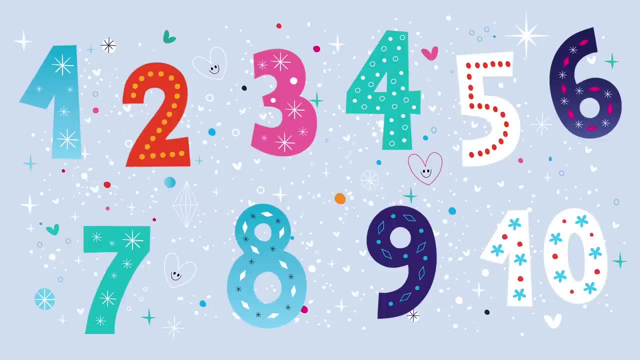 Gently open your eyes and have a stretch, Take a moment to just relax, Just sit. How many counts did you manage? Maybe you made it to ten, Maybe you did a few sets of ten. Whatever you managed, you did really well. 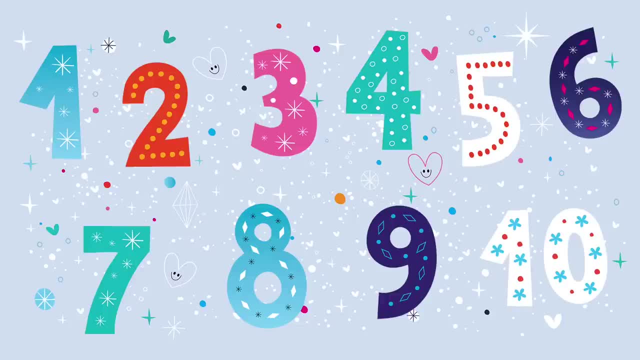 Your brain is a busy place and this practice will help it become so much calmer. I look forward to seeing you here again soon. This is Jamie saying peace out.